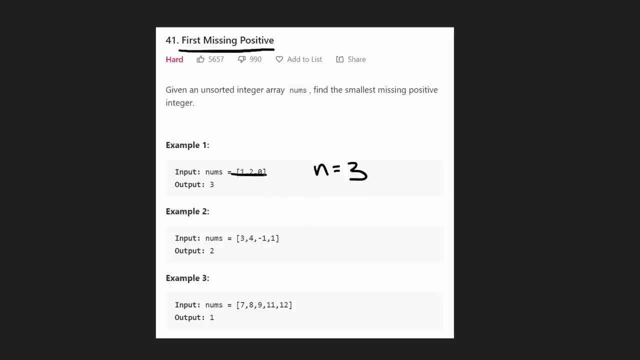 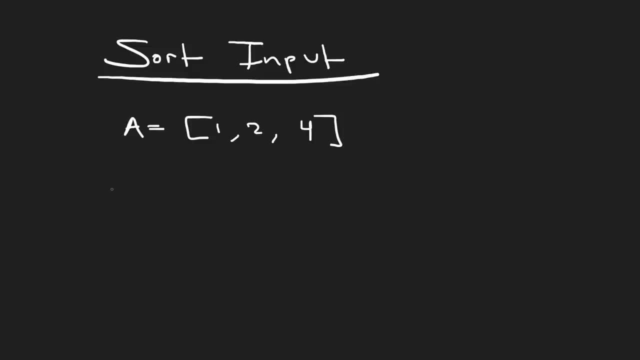 not a three, so we don't care. So now we've run out of the array. What's the smallest missing positive integer Three? right, We were keeping track of that, so we're going to return three. So basically, the way I was going through the problem right now is one way you could solve it. 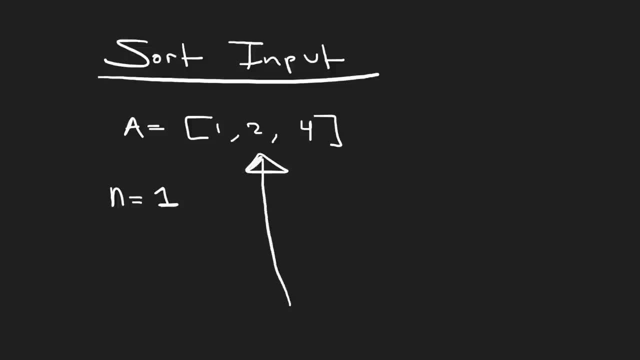 but to solve it in that way, you would need to sort the input array in ascending order. So we're going to sort of be greedy here, right, We're just going to say one is the smallest positive integer. that's missing, right? And since we know our input array is sorted, we know that. 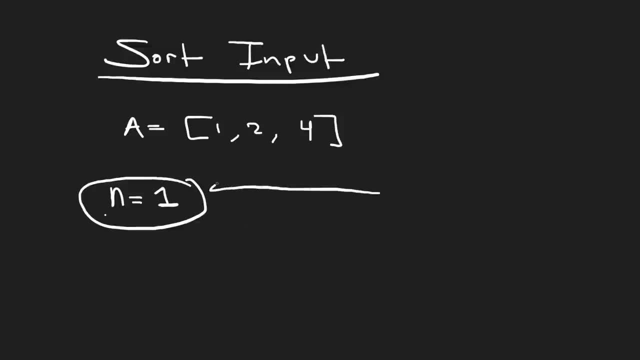 if there exists a one, then clearly we were wrong in our assumption, right? So in this case we do see a one, so we were wrong. So then we'll change what our solution is to a two, right? And then we'll see a two, and then we know we were wrong again, right? So then we're going to change. 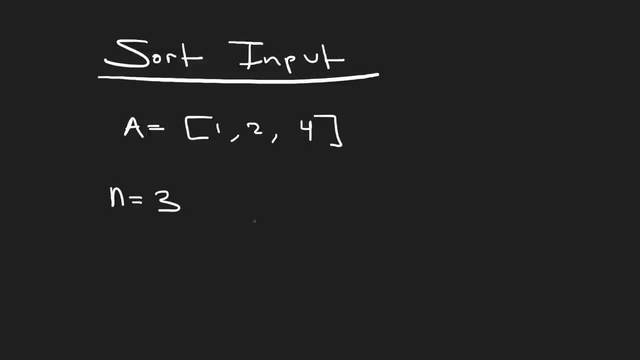 our answer to a three. We're going to say, okay, maybe three is the smallest missing positive integer, and then we're going to get to a four, right? And so once we've gotten to a four, we know every value that's going to come after. it is going to be greater than or equal to. 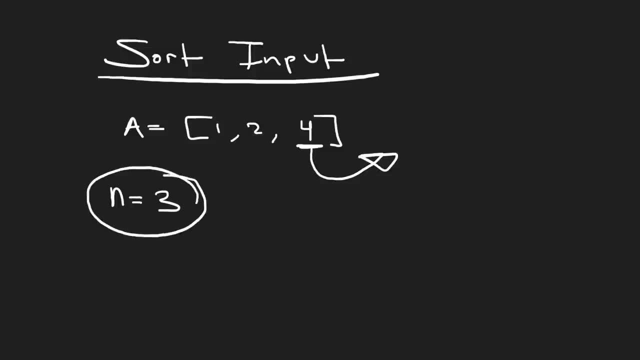 three. So at that point we basically know: yes, three was the one that was the smallest missing positive integer. Now the time complexity is going to be n log n, because we are sorting this input array. But one thing to notice with this is see the size of our input array, The 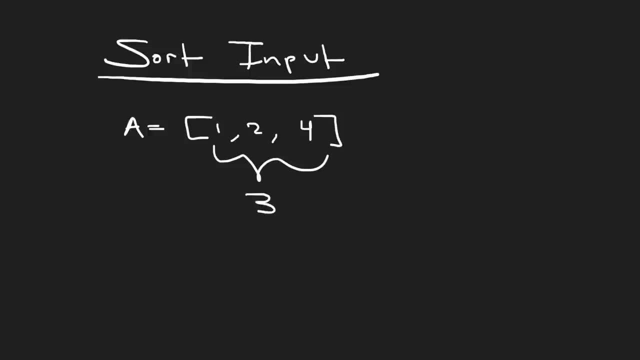 size of the input array is three, right. So that means in the worst case, the smallest missing positive integer in the worst case, right In the largest it could possibly be, b is going to be four. Why is that? Why is it going to be four in the worst case? Well, 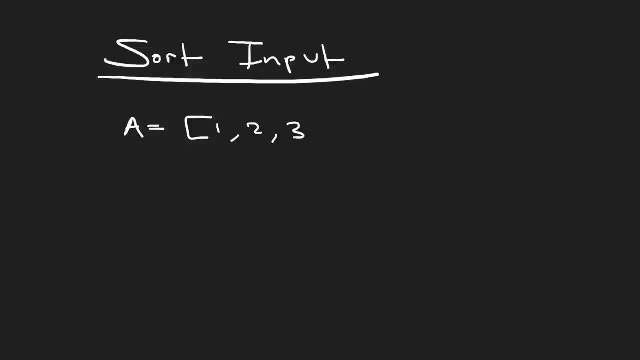 take a look at this. What if the input array we got was one, two, three, right? Remember, the size of our input array is limited to size three. So in this case, if we had one, two, three, then we know that n would be four. the result would be four because we're missing the smallest. 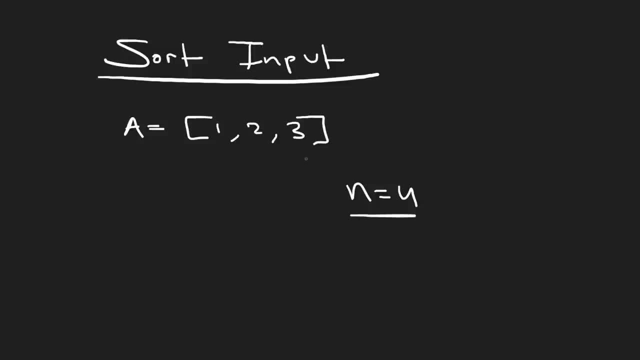 positive integer we're missing is the four that would go here right. If, for example, we did not have all three of these right, Maybe we're missing that three- like we had previously, then we would have the n equals three right. Or for example: 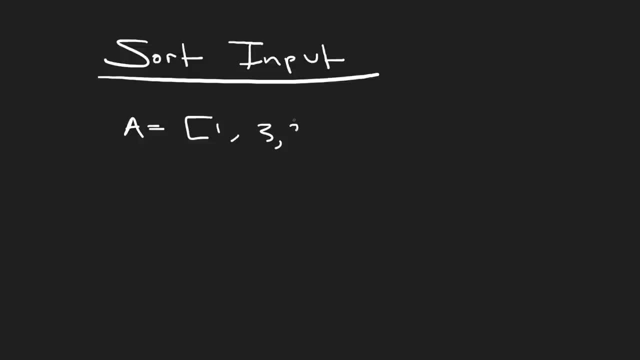 maybe we would be missing a two, right? Maybe we have one, two, three, four, then in that case we'd have a two that goes here, right. Two, three, four, then in that case the smallest missing is: 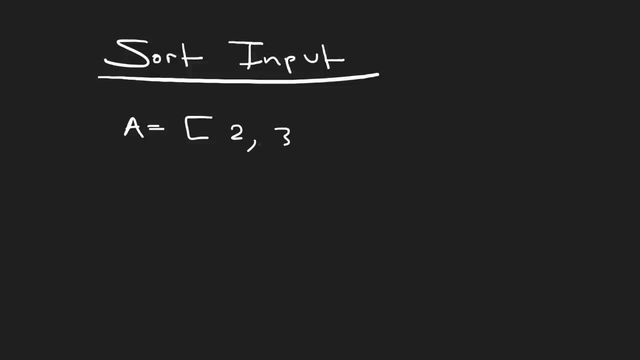 going to be one, But basically, no matter how you arrange this right, maybe we would just have really big integers, for example, 10, 11, 12.. What's the smallest missing in that case? Again, that's just going to be n equals one, right? So basically. 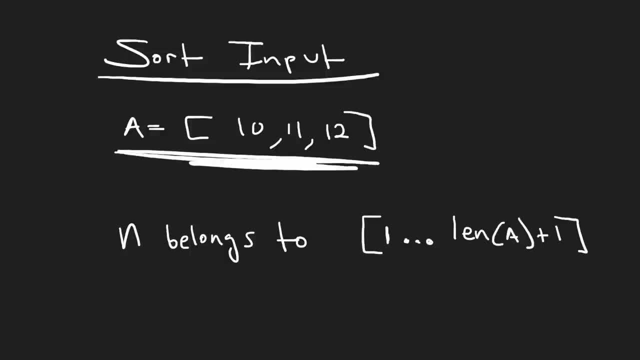 what I'm saying here is: no matter what our input array is, no matter what the values go in it, the answer, our result n, the smallest missing positive integer is going to belong to the set between one and length of the array plus one. That's pretty obvious, right? That's mathematically. 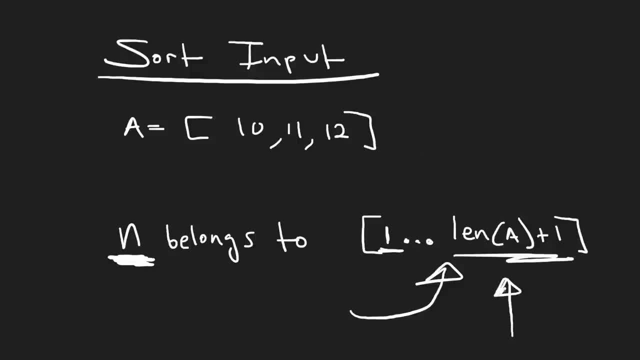 obvious right. We could not have a smallest missing positive integer that would be larger than this. if our input array is just, you know, limited in size, We could not have, you know, a missing positive integer. So this is our solution, set right And we're given that. 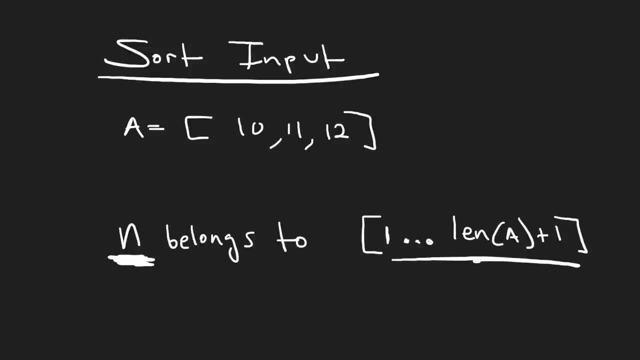 based on the length of the input array. So in reality, we actually don't need to sort this input array. We can actually take the input array, convert it into a hash set. Why are we converting it into a hash set? Because we're going to brute force this. We're going to go through every single. 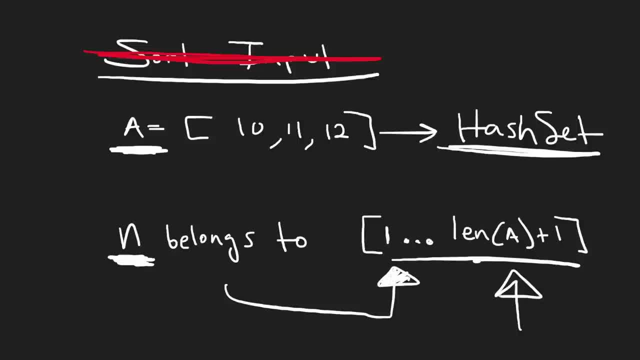 value from one to n plus one right, Or the length of the array plus one. So we know the solution belongs to this. We're just going to have a for loop that goes through all of these values, tries each of them right. So for example, 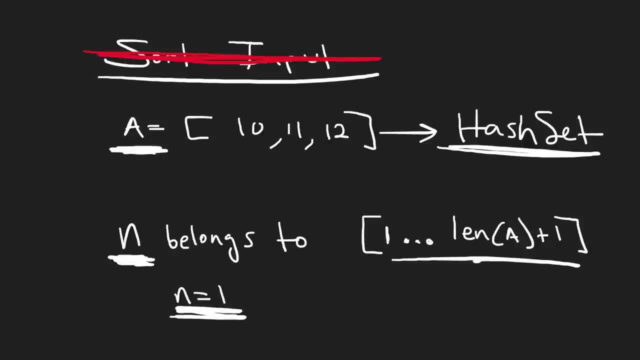 we're going to try first. we're going to try n equals one. We're going to check: does n equals one exist inside of our hash set And we can check that in O of one time, right, If it does exist in? 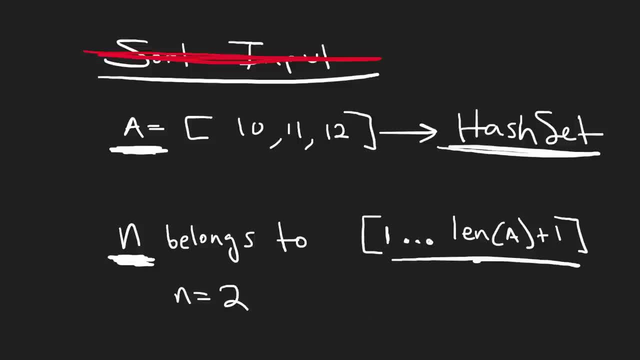 our hash set, then we're going to try n equals two, right? If that doesn't? if that exists, then we're going to try n equals three. So if n equals three, for example, does not exist inside of our hash set, then we're going to return n equals three as our result: the smallest missing. 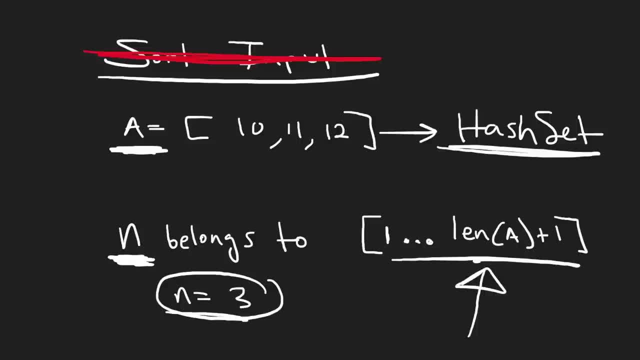 positive integer. If, for example, we go through the entire loop and we don't find any value. So, for example, if we tried, the n equals the length of the array, and even that was found in the hash set, then by default we're going to return: n equals the length of the array plus one. So we're 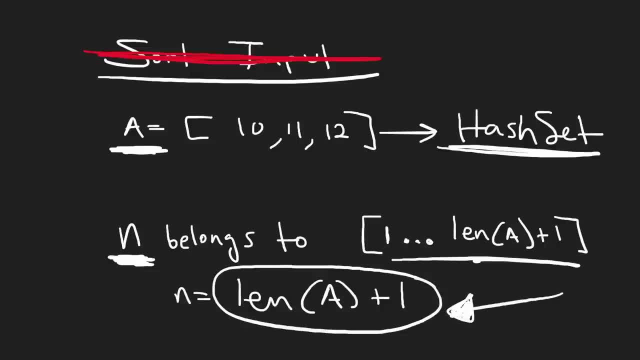 this is our worst case scenario. This is the largest it could possibly be, And so, since each of these operations just takes O of one time, and we're doing it for every value based on the length of the input array, this is going to be one times n. that's just big O of n time complexity. But 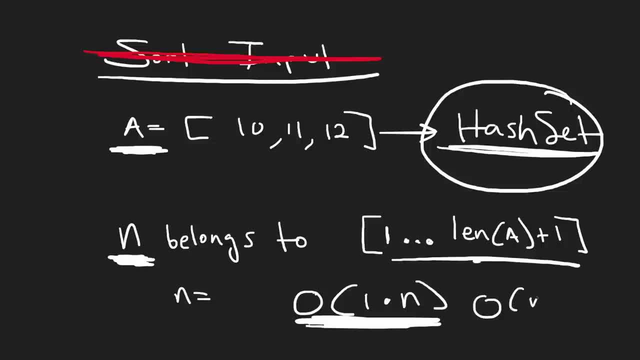 the hash set is taking extra memory right, So that's going to be big O of n memory as well. But we can use this to our advantage. We can devise a way where we actually don't need a hash set. How can we do that? Well, we are going to need some extra memory, But it turns out we can. 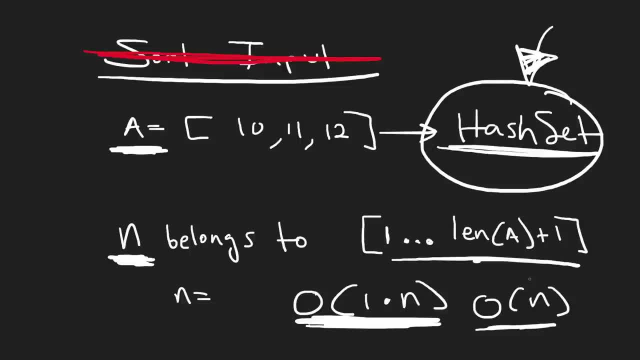 use this input array as that extra memory, So it doesn't actually count as extra memory. So we can take this time complexity or this memory complexity, big O of n, and reduce it all the way down to big O of one by using the input array as our extra memory. So, like I said, we're going to 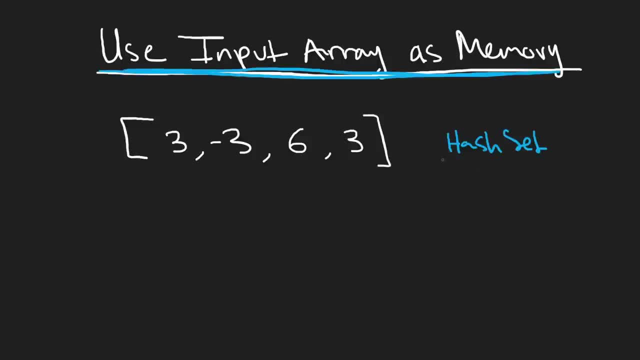 be using the input array as extra memory. just like we used a out, like an extra memory hash set, we're going to be using our input array as a hash set. How am I going to do that? Remember how our solution set is basically from one all the way to the length of the array plus one right. 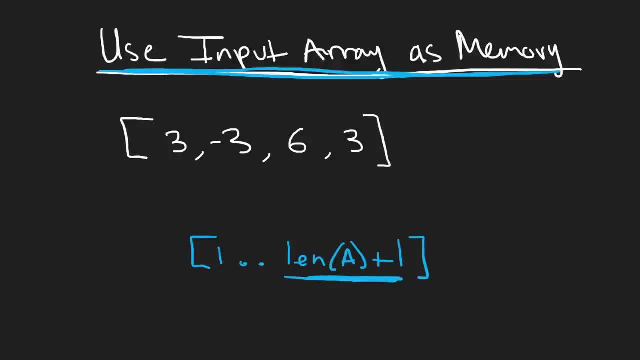 This is our solution: set between one and the length of the array plus one. So for every value between one and the length of the array, right, we have an index for that right. So one is going to be mapped to the zero By Dr. 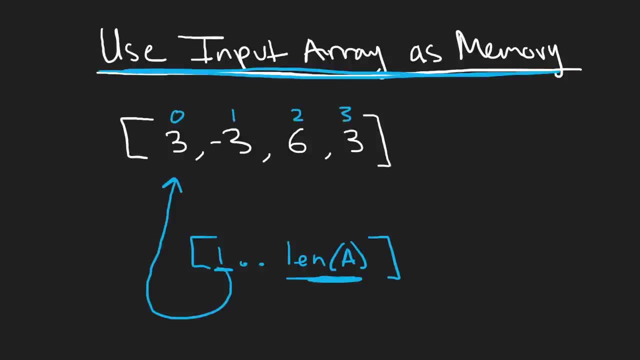 Dr right Zero index one index two. index three. index right. The last value, length of the entire input array, is going to be mapped to the length of the array minus one index right. So in this case we can see the length of the input array is four. So four minus one is going to take us. 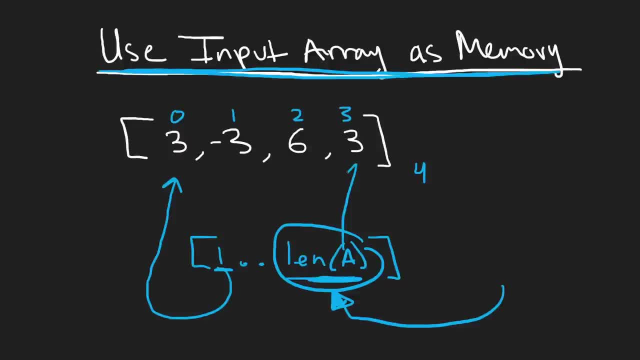 to this index, right? So each of these values has a position in the input array. So how am I going to use the input array? basically to tell us, for example, if I want to know in constant time if the value two- right, the value two does two- exist in our input array, How can I know that in constant? 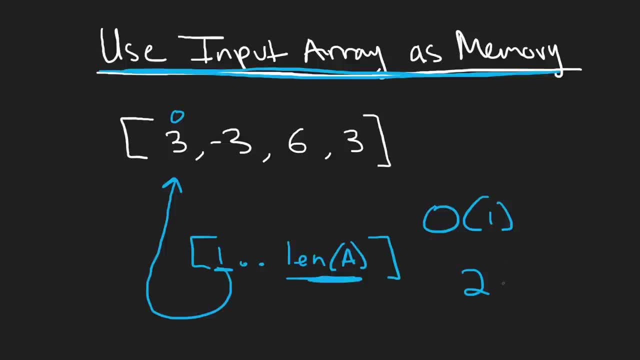 time. The way I'm going to do it is I'm going to say: okay, we want to know if two exists. I'm going to take two minus one, right? That's going to give us our index value. I is going to be two. 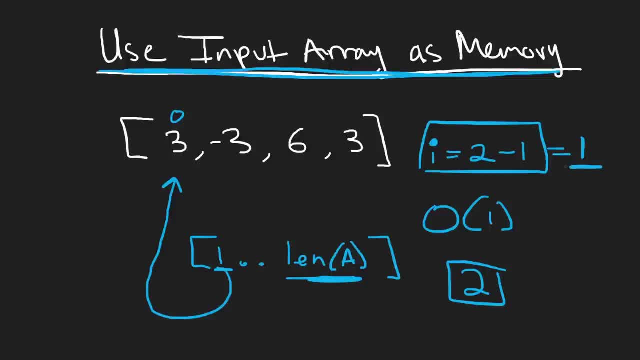 minus one. We know that evaluates to one, So we're going to go to the one index right which is over here. This is zero, This is one, And we're going to go here and we're going to check: is this value? 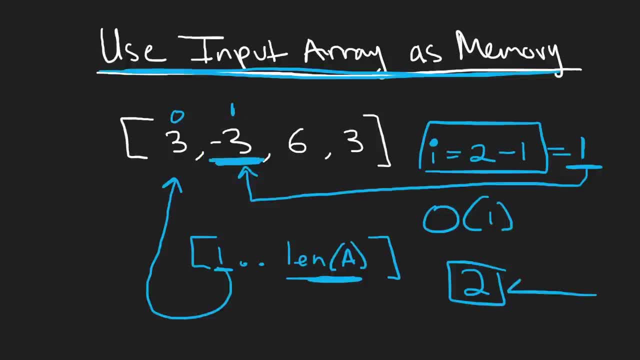 negative. Negative tells us that two exists in our input array. We don't know where it exists, but we know that two does exist. We can figure that out in constant time, right? So we're going to use negatives to determine that. Just one problem. It turns out that this: 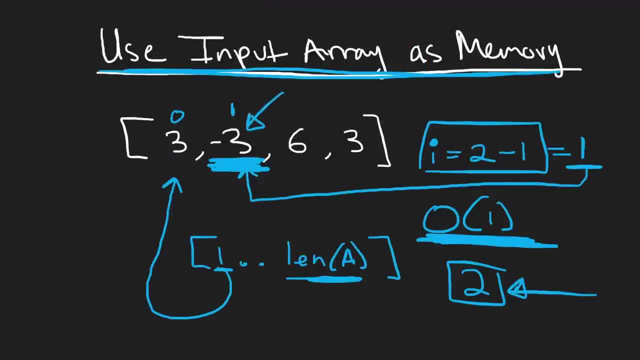 input value is two, So we're going to take two minus one, right? So we're going to take two minus one. So we're going to take two minus one, right? So we're going to take two minus one. And the input array that we're given can have negative values by default. So how am I going? 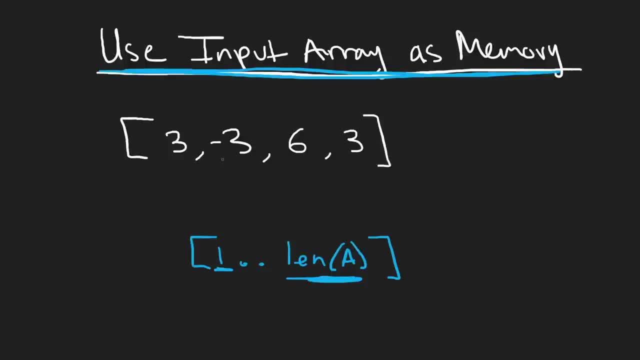 to handle that. Well, it turns out, we're looking for the smallest missing positive number. Obviously, by just looking at this, we know that that's going to be n equals one. That's going to be the result, right. But we're looking for an algorithm to solve this problem And it turns. 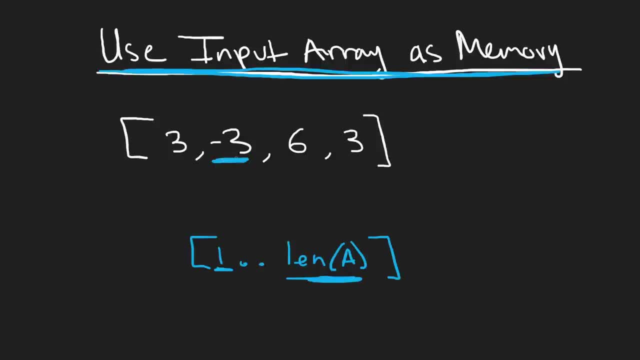 out that negative numbers are useless to us. We don't really care. If I took every negative number inside this input array and just crossed it out, it would not matter, right? So that's exactly what I'm going to do: I'm going to take every negative number. for example, 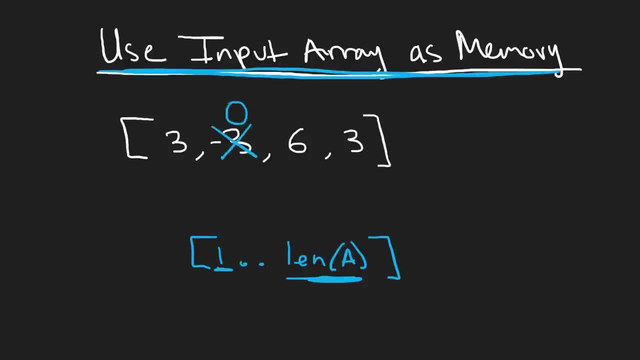 negative three. get rid of it. replace it with a zero. Why am I doing a zero? Why don't I just replace it with a one right? Well, in that case, if I replace it with a one, I just changed the. 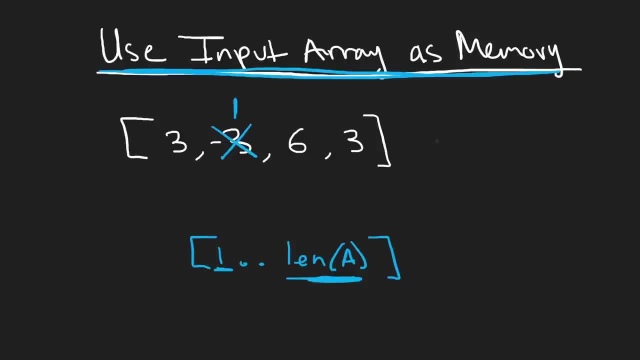 entire input array, right. Remember, the solution to this problem is n equals one. If I add a one to this, then I've changed the solution to n equals two, right? We don't want to do that. That's why we're giving it a neutral value of zero, right. I'm replacing every negative value. 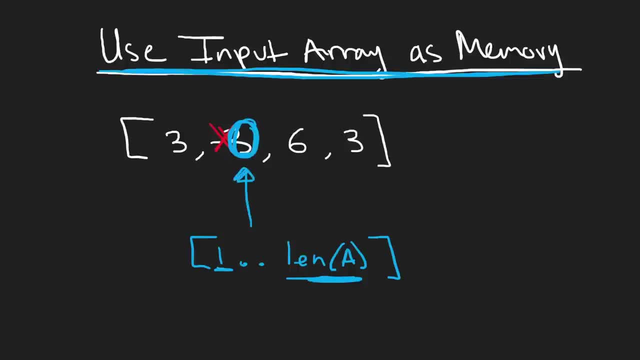 with a zero. So it might be a little messy, but let's just assume that this has been changed to a zero. So we're going to basically scan through the entire array, change every negative value to a zero. We can accomplish that in O of n time and we're actually going to be needing to scan. 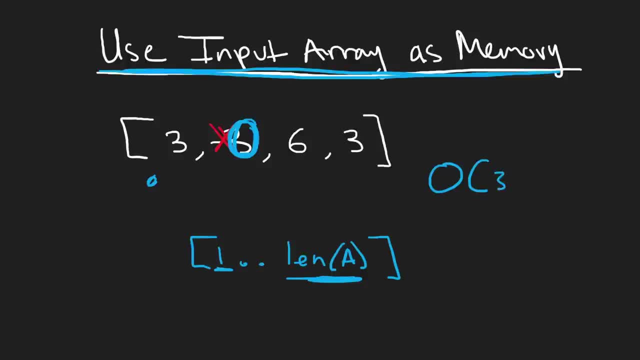 through the entire array two more times, So it's overall going to end up being three times n. but that's still linear, right? That's still going to reduce to big O of n And since we're not using extra memory, we're using the input array as extra memory. 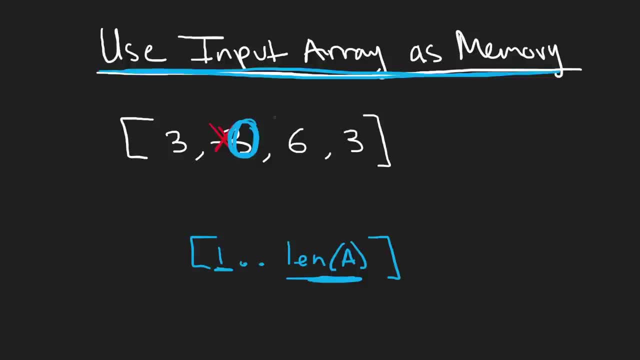 Overall, memory complexity is going to be big O of one. So now, what I'm going to do is I'm going to start at the beginning of the array again, and now is when I'm going to start marking values as appearing in the array, For example, three. right, We have a value, three- We want to mark. 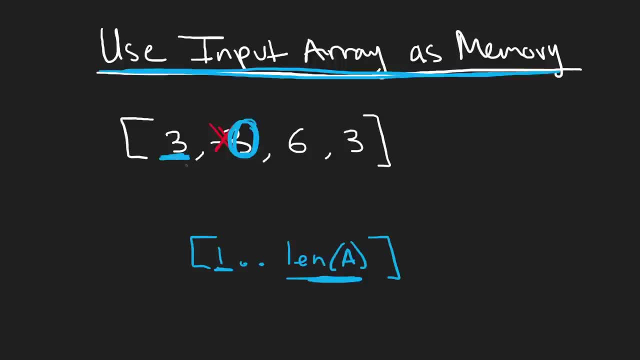 that three exists in our input array. So what we're going to do is we're going to go to the index. i equals three minus one, That's index two. Index two is over here, right, And we're going to change this value to a negative value. 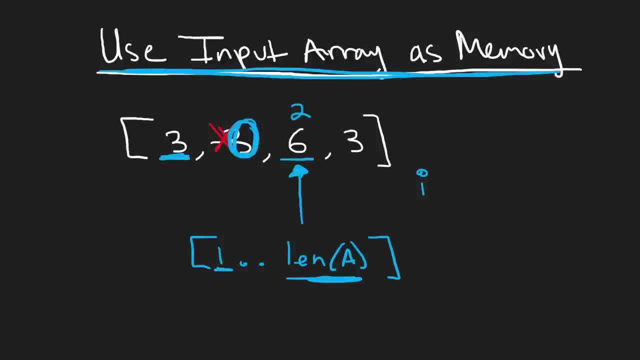 If it's not already negative, right. Right now we see that it's positive, So what we're going to do is we're going to change it to negative, right, So we're just going to add a negative sign. This is going to be negative six from now on. right, So we are changing values, right? So it. 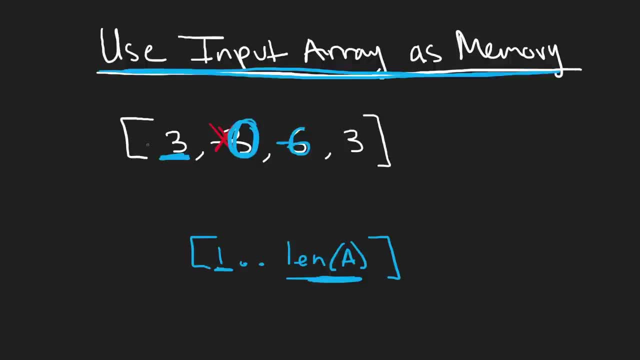 turns out that it's possible that this also could have been a negative three right. So basically, every time we get to a value, we're actually going to be taking the absolute value of it, So absolute value of three- and then minusing one to find the index. 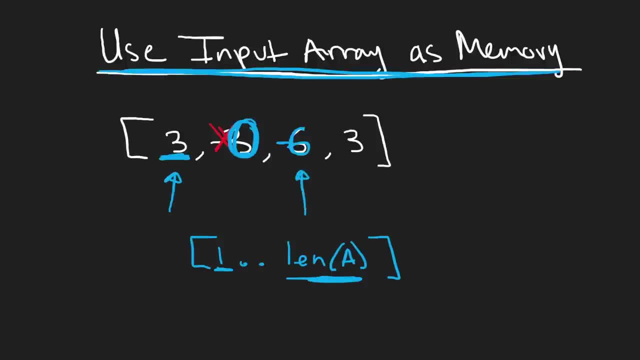 So, since index two is negative, we know that three exists in our input array. Next, we're going to go to this value. It's zero, right, It turns out i equals zero minus one. That's going to be negative. one, right, That's out of bounds of our input array. right, That's going. 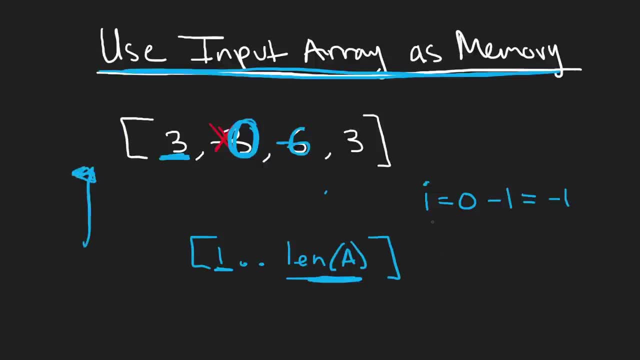 to be over here, right? That's out of bounds. So we're not going to be filling values that are out of bounds. So it turns out this is out of bounds, We're not going to fill it. Next we get to the 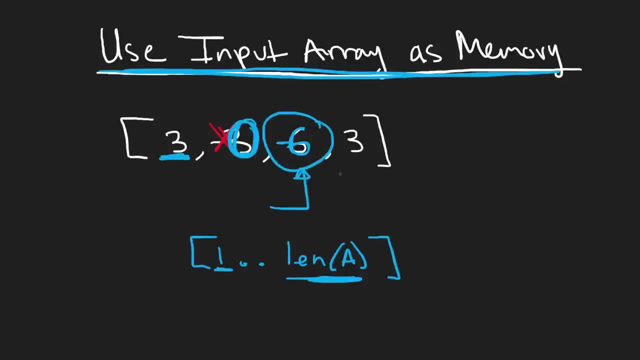 value six. But remember this is negative six now because we changed it, So we're not going to be taking the absolute value of this. Absolute value of negative six is going to be six, right. So we're going to get i equals six minus one. That's going to be five, right. So again, we went out of. 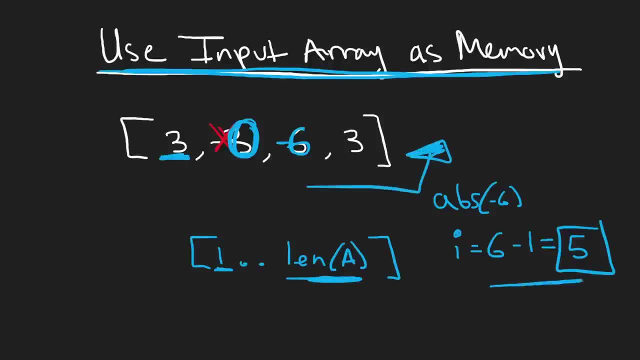 bounds right, That would be somewhere over here, but that's out of bounds right And we know this would never be the solution anyway because it's too big. So okay, and then we're going to go to the last value. Again, we found a three right, So we're going to go to. i equals three minus one. 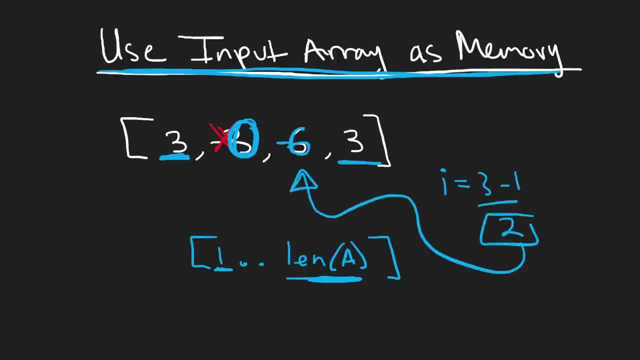 That's going to be two. We know index two It's going to be over here And we're going to change this to a negative. But good thing for us, it's already negative. If it's already negative, we don't want to change it back to a positive. 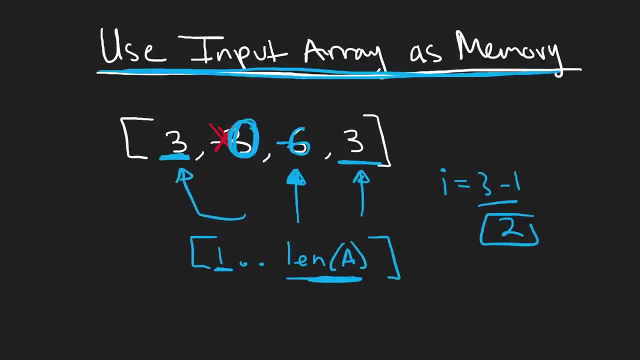 number because, remember, three does appear in our list. Just because it appears twice doesn't mean we want this to be positive. We still want to know, in constant time, that a three exists in the input array. So we leave it negative. So then, one last time. we're going to be iterating, not through. 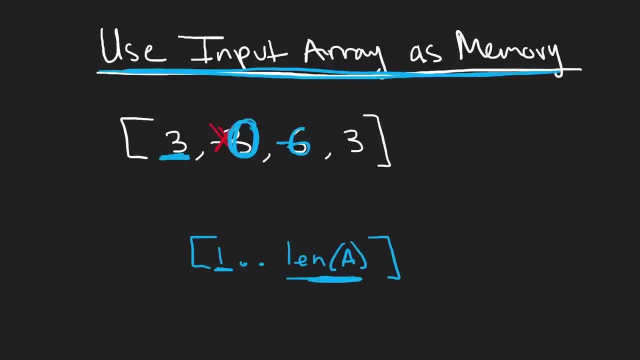 this loop. Now we're going to be iterating through this set, So we're going to be iterating through one, through the length of the input array. a right, So that's also going to be an O of n operation, right, Basically the length of this input array. So we're going to start for. 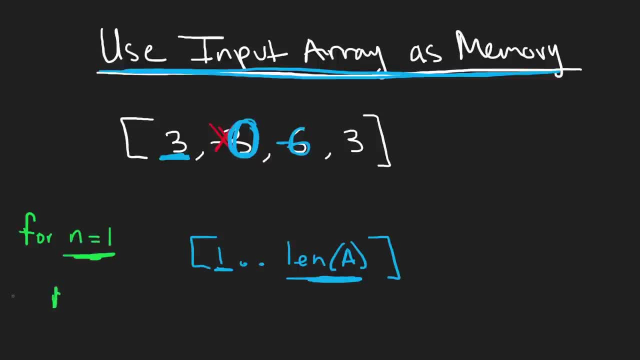 n equals one, right, We're going to take one. We want to compute the index, right, So we're going to take one. minus one is going to be zero, right, So we want to know: does one exist in our input? 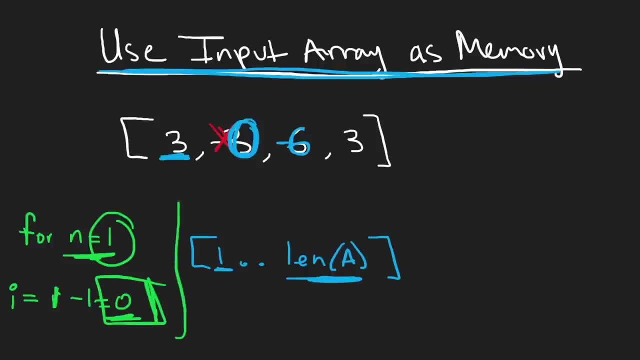 array. We can check that by checking the zeroth index of our input array. If it's negative, that means one Does appear in the input array. If it's positive, which in this case, it's positive, right, This is. 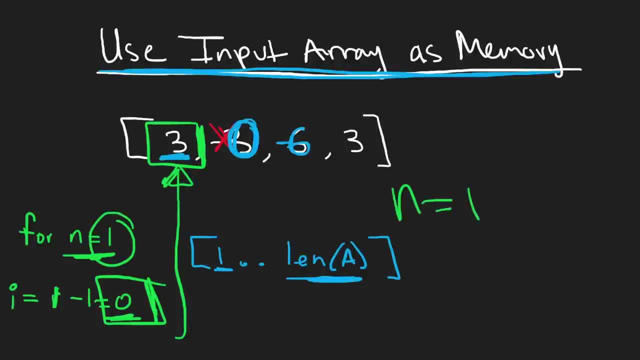 positive three. That means n equals one does not appear in our input array, right? Therefore, n equals one is the smallest positive integer that does not appear in our input array. Awesome, right? That's the solution. We did that with three loops, but it still ended up being big. 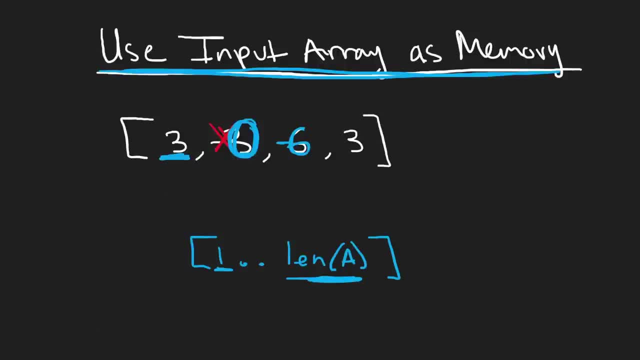 O of n. There's one last edge case that I'm going to show you. Notice how this value was originally a positive Six, right, But we changed it to a negative six because we still wanted to know what value was originally stored here. right, So we could take the absolute value and then convert it to a positive. 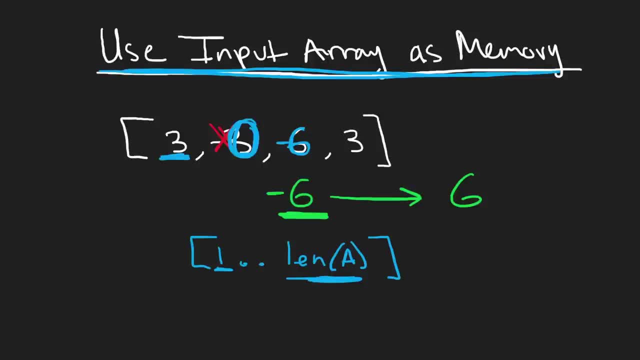 six. right, We wanted to know the original value, but we also wanted it to be negative so that we could indicate that a positive three exists in our input array. right, But my question to you is: what if the value that we're changing? for example, what if we had one more value in our input array? 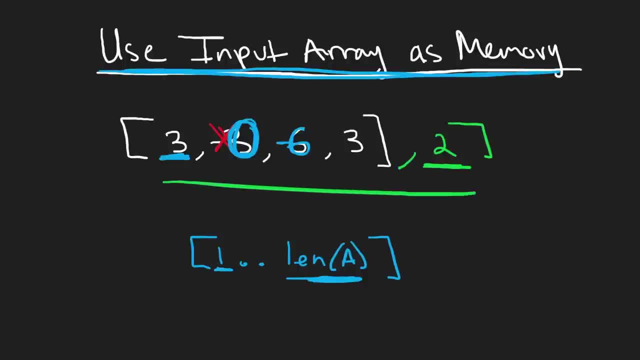 and it was a two, Then we want to mark that two exists in this input array so we can compute: i equals two minus one. That's going to be one. So we're going to go to the one index value in our input array, right This? 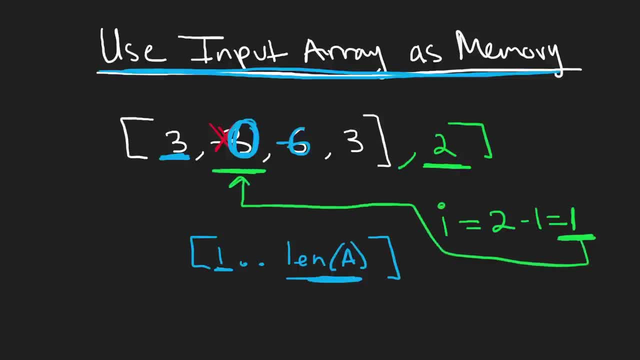 is index zero. This is index one right. So now we want to mark that this, that we want to change this to a negative value, to mark that two exists in the input array. Hold on: This is a zero right. But we don't like changing the value, We just want to multiply it by negative one. 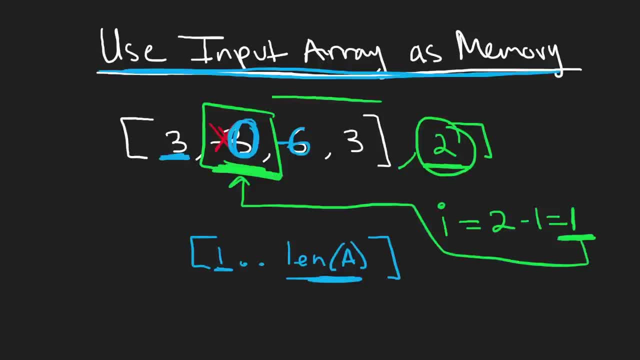 but it'll stay zero. So what value can we change this to? For example, if I just change this to a negative one right, a negative one value, we can't do that. Why can't we do that? Because then we're changing the. 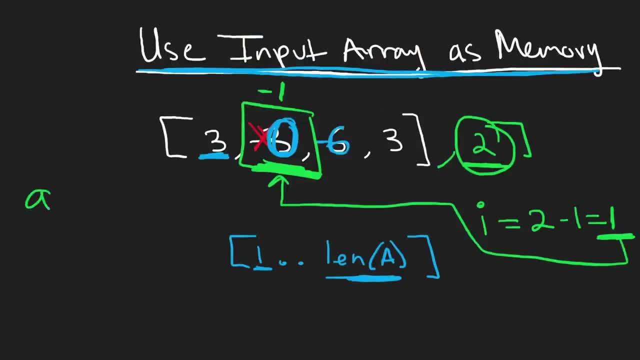 input array. Remember this negative one will. eventually we're going to take the absolute value of the negative one right. And then basically we're saying we're assuming that a one exists in the input array, But originally there never existed a positive one in the integer. 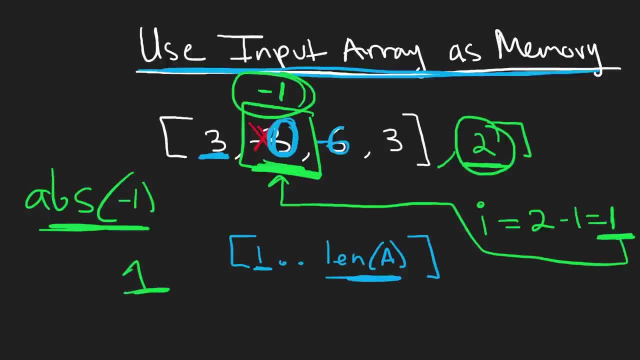 array. So we can't do that. So we're going to change this to a negative one, right, And then we can't change this to a negative one. If we do that, we change the solution of this input array. So we have to change it to a negative value. that does not affect the solution, But remember. 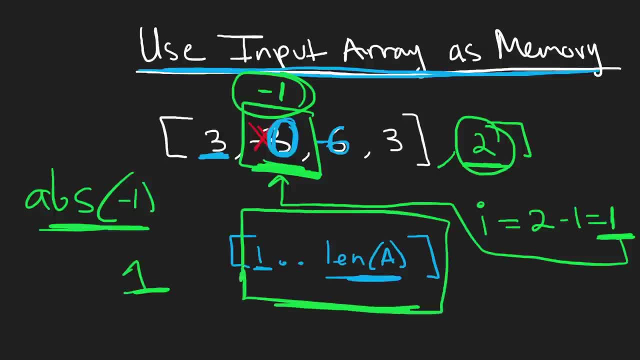 the solution set could only be from one to the length of the input array. So if we change it to supposedly negative- length of the input array plus one right- so basically we're taking length of the input array plus one right. so basically we're changing it by negative right If we do that. 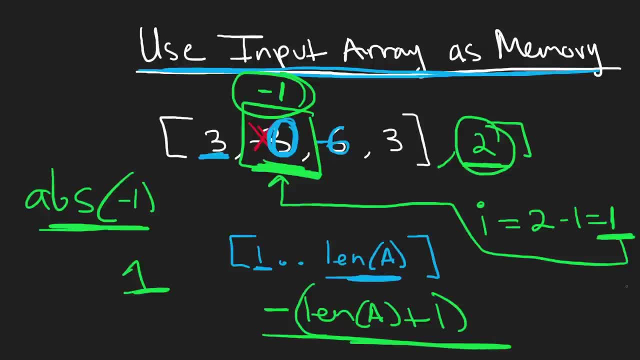 we're not changing the solution set right. Well, actually, technically, this could be a solution right. This would be the worst solution that it could possibly be. the greatest value could possibly be. But notice, with this value, it's out of bounds when we, when we compute the index of it. 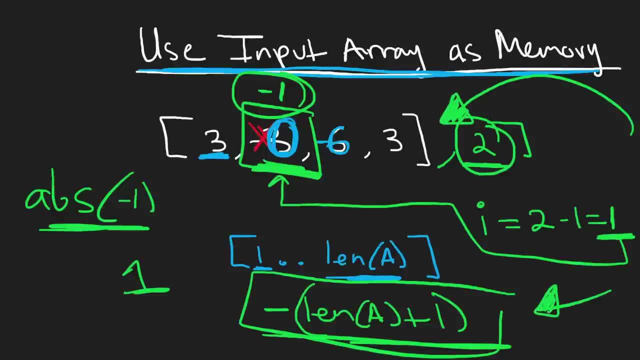 So, basically, this is a good default value to give it, because we're never going to be marking. that value is showing up in our input array because it's always going to be out of bounds. That's basically the point that I'm trying to make. So if we do that, we're not changing the solution set. 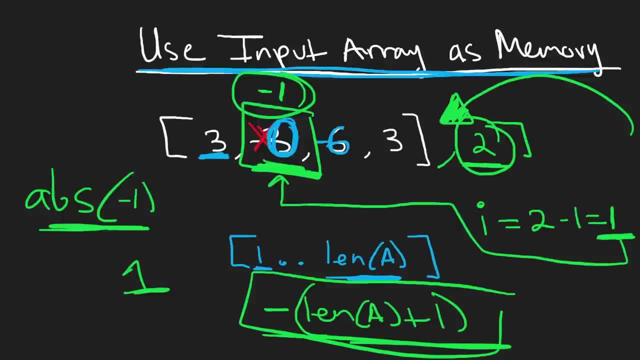 trying to make so that basically handles all the edge cases. So if we found a zero, this is the negative value that we would give it to. Otherwise, we would just take that positive value and then multiply it by negative one. So with all those edge cases being said, now let's actually jump. 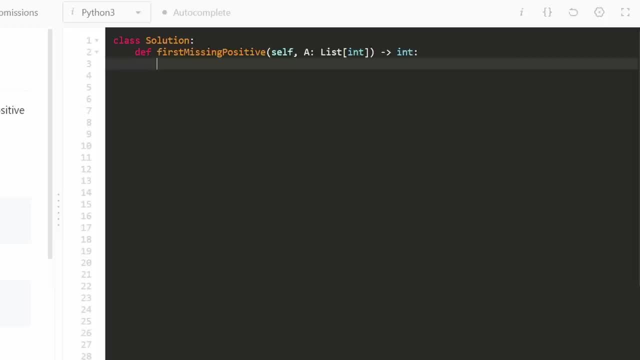 into the code. it's going to be three linear time loops, So remember, the first thing I'm going to do is go through every value. And, by the way, I changed the name of the input array to a just because it's shorter. we're going to be writing that a lot. I don't want to change it. I don't. 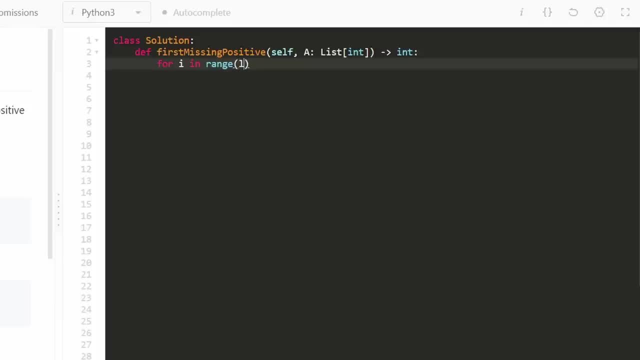 want it to be nums because I don't want to type that a lot, But I want to go through every single value. So, for range of the length of this input array, if the value at that, at that index, is negative- remember if it's less than zero. 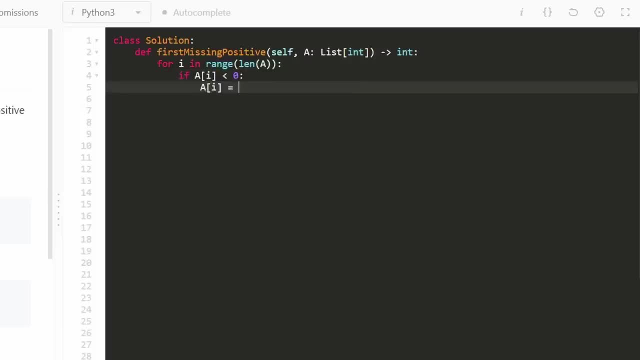 then we're just going to change it to be zero. that's a good default value to neutralize these negative values to. the next portion of this algorithm is going to be another for loop just iterating through the input array. But this is the part where we're marking if a value exists. 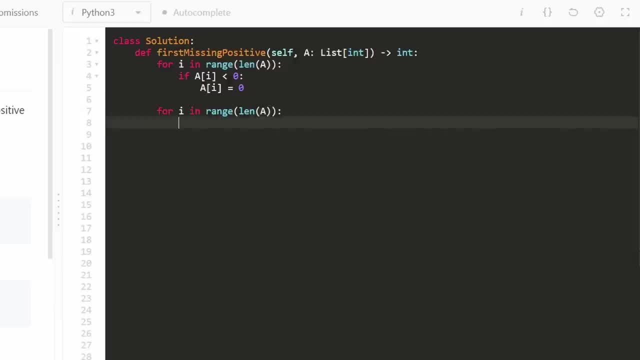 in the input array or not. So we're overwriting the input array a, but remember we're only doing that for values that are inbound. So basically, what I'm going to say is if, what if our value at a, at position i, index i, is between one or the length of the input. 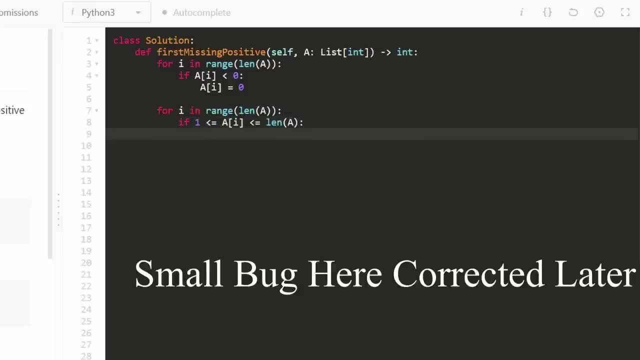 array a if that's the case. so if this is the case, that means it's inbounds. but we it could technically possibly be negative Because as we're going through the loop we know we're going to be changing values to be negative. So we're going to take the absolute value of that. So absolute. 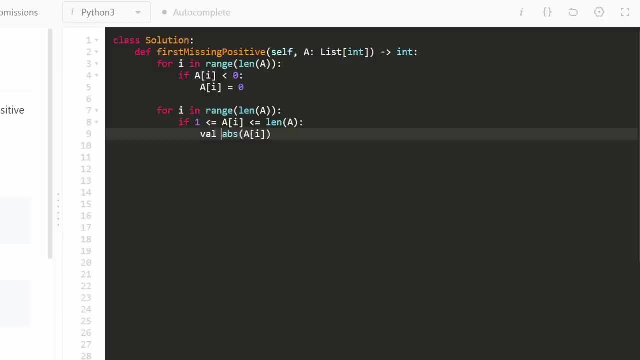 value of this and we're going to store it and let's say value next. So we want to overwrite a position right. So, for example, we want to say a of value minus one- right, because we were taking the value subtracting one to get the index right. So what we're trying to do is mark that, this value. 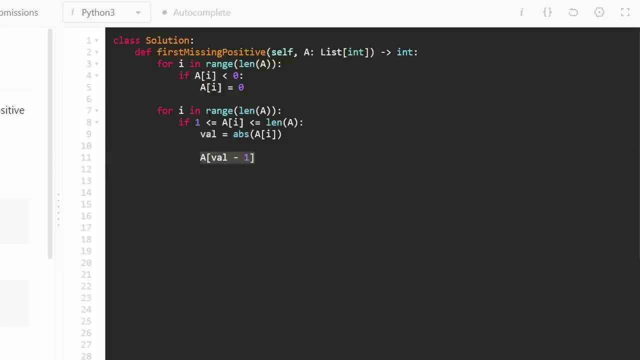 exists. we're doing that by taking this and creating it to be negative. So what we're going to do is basically say, multiply this by negative one. But remember, we're only going to be doing that if this value is originally value minus one if it's positive. 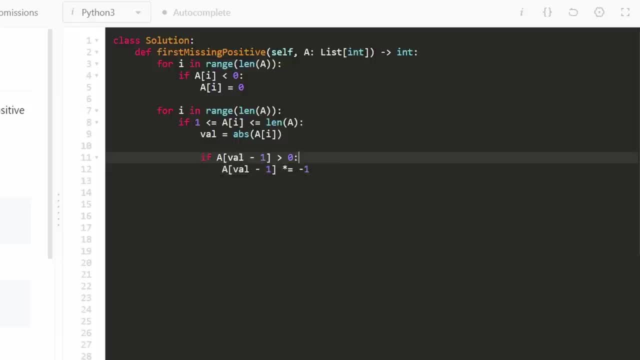 right, if it's positive, then we want to make it negative. if it's negative already, then we don't need to do anything. But the last case was else. if this value happens to be zero, right, that was the edge case that we were worrying about. So if this happens to be zero, then what we can do is assign. 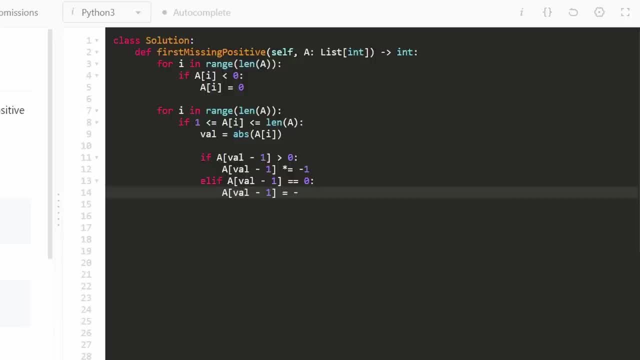 it to a special value of negative one. So if we want to make it negative, then we want to make it negative, right? So? so let's look at the result of this. So, instead of using a hash set, we use the. 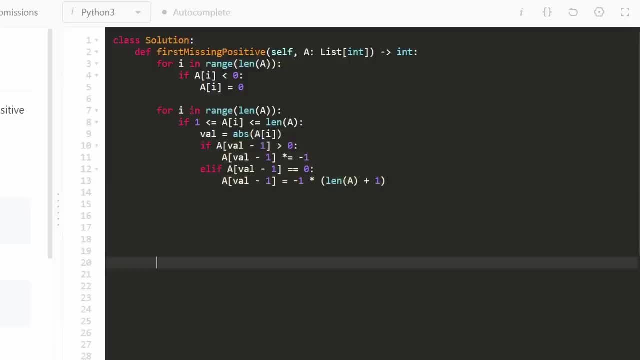 input array to doing this integration and into the array. so equal to zero. So we get negative one multiplied by the length of the array plus one, And that's actually this entire loop. So once this loop is done, we have basically, instead of using a hash set, we basically used our input array to. 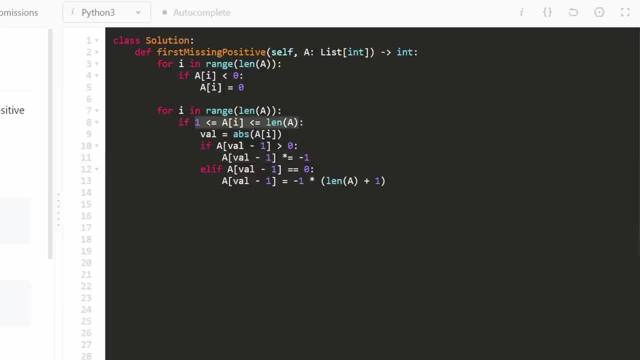 mark which values between the range one to the length of the input array have been do appear in this array. So now we actually want to determine what the solution is. So I'm going to say for i, in range from one to the length of the input array, maximum of one. this array m can cut to the length. 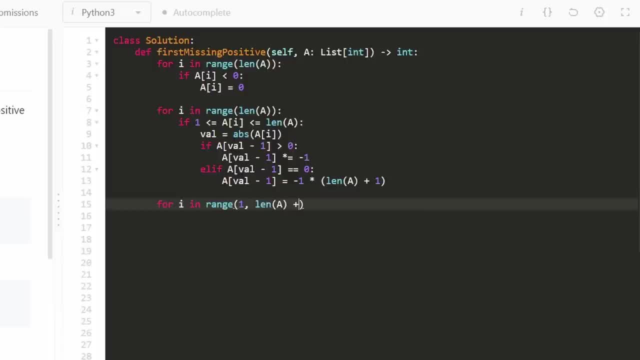 of the input array. So that's the answer. Now we can actually say, okay, so there's this little length of the input array plus 1.. Now we want to know: if i does not exist in the input array, How do we know that If a at index i minus 1, remember. so for any value we're subtracting it by 1 to. 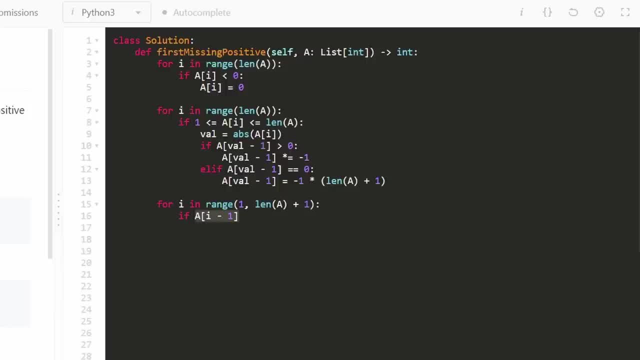 correspond to the index. So if this happens to be negative, that means this value does appear. If it's positive, though, or 0,, if it's greater than or equal to 0, that means i never showed up in the input array. That means i was the smallest positive integer that did not show up because